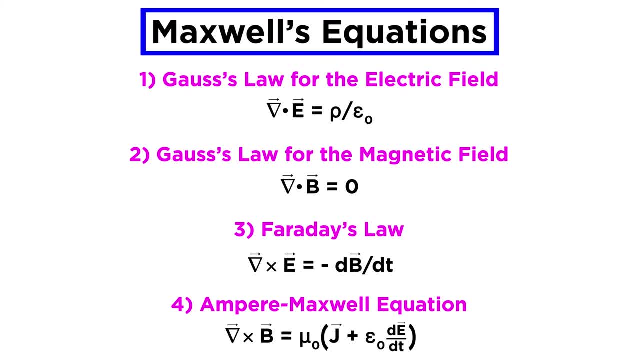 understanding of the universe. We will begin this next phase of the series by examining Maxwell's equations. We have mentioned these in passing, but we did not examine them with any rigor. This is because a proper treatment of these equations requires fairly advanced mathematics, even beyond basic calculus. Those who wish to move forward with this series. 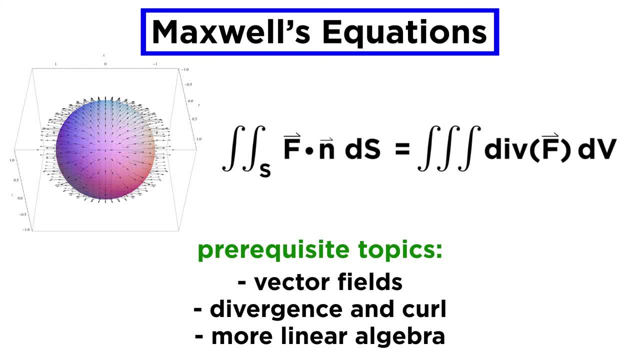 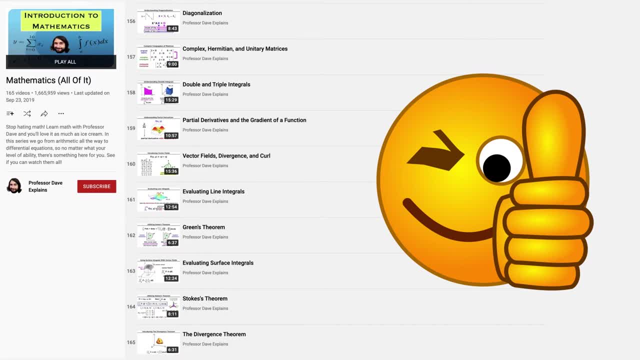 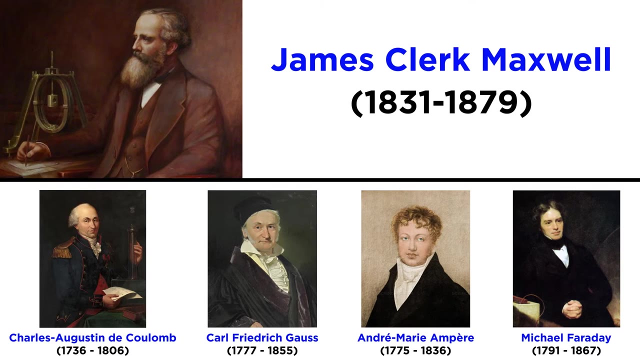 will need to understand vector fields, divergence and curl and other topics in linear algebra. Fortunately, I have covered all of these in my mathematics series, so if you feel that you want to move forward with physics, please do so. Maxwell's equations for electromagnetism elegantly correct and combine almost a hundred. 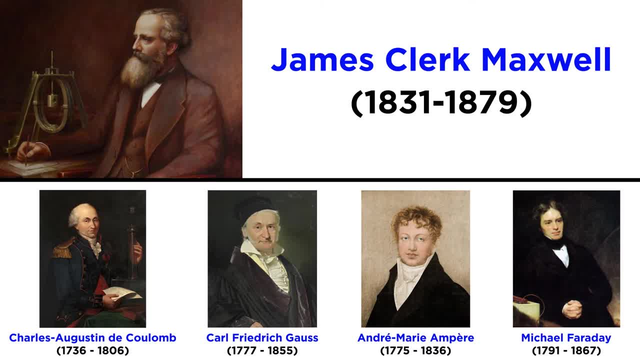 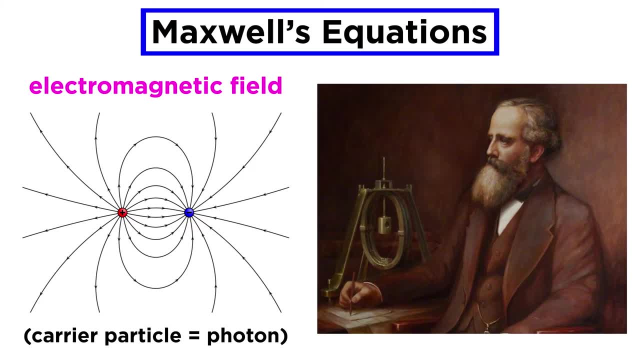 years of work by earlier well-known scientists, those being Coulomb, Gauss, Ampere and Faraday. Formulated almost two hundred years ago, they are still the simplest way to accurately represent laws of the electromagnetic field and its carrier particle, the photon. Each of these 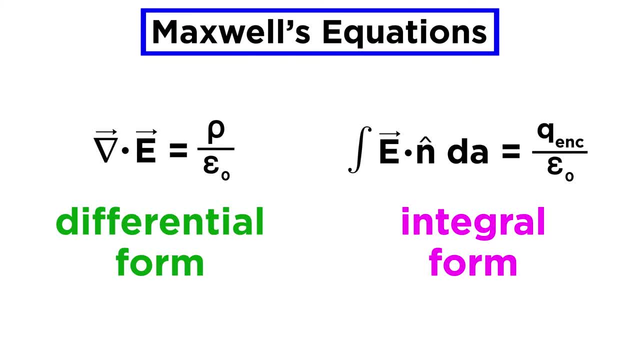 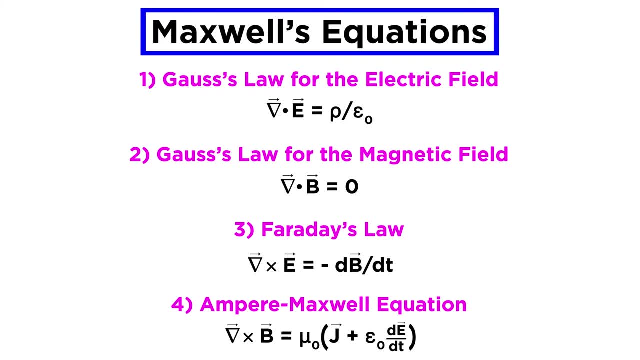 four equations, has two forms: a differential form and an integral form. We are going to examine Maxwell's four equations, one at a time, over the next four tutorials. The first one is Gauss's law for the electric field. so let's start with the foundational concepts. 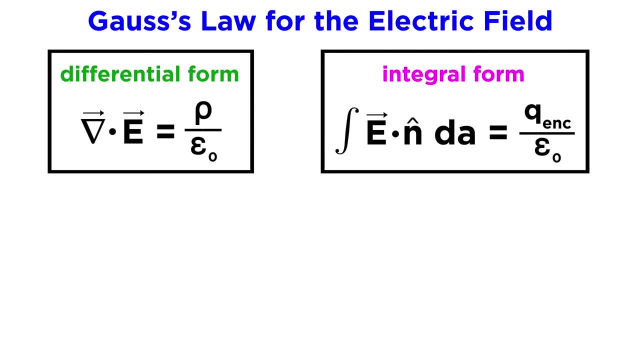 behind the derivation of this law. As we mentioned, this law has both differential and integral forms. These two forms are called differential and integral. The differential and integral forms are useful in entirely separate situations. The differential form states that the divergence of the electric field in a given region is related to the charge density within that. 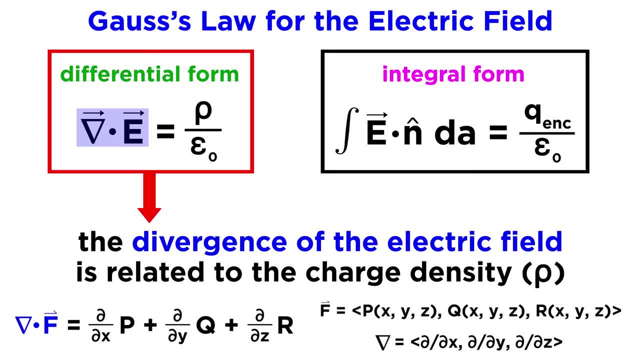 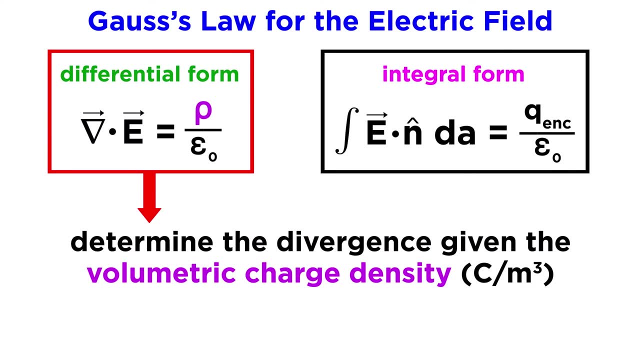 region. Remember that divergence means we are finding this dot product where the del operator is a vector comprised of the relevant partial differential operators, and that the divergence of a vector field, like this electric field, gives us a scalar field. The differential form states that the divergence of the vector field is related to the charge density within. 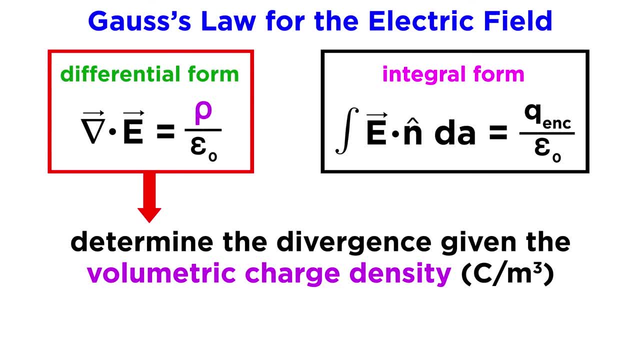 that vector field. This form is used to determine the divergence of an electric field at a particular point if the volumetric charge density rho is known, meaning the quantity of charge per unit volume measured in coulombs per cubic meter. Epsilon naught is a constant representing 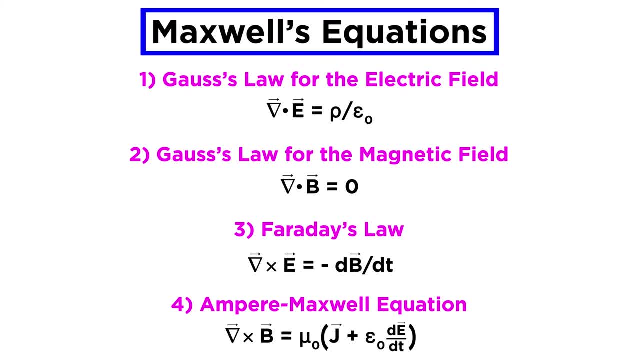 understanding of the universe. We will begin this next phase of the series by examining Maxwell's equations. We have mentioned these in passing, but we did not examine them with any rigor. This is because a proper treatment of these equations requires fairly advanced mathematics, even beyond basic calculus. Those who wish to move forward with this series. 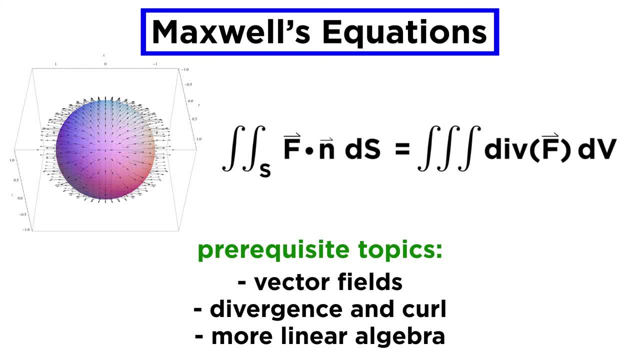 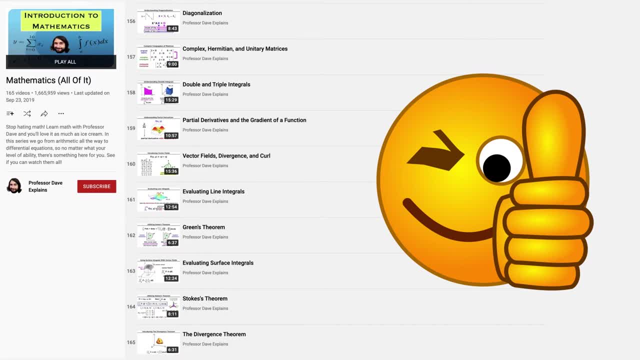 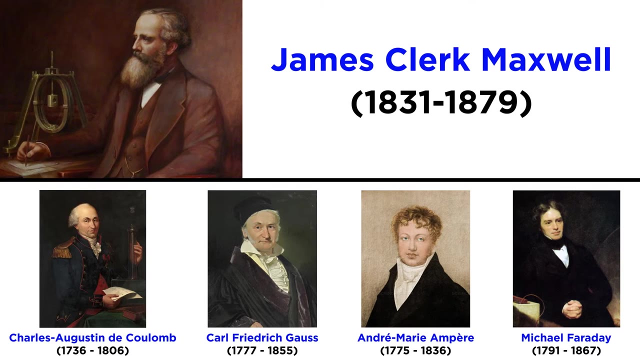 will need to understand vector fields, divergence and curl and other topics in linear algebra. Fortunately, I have covered all of these in my mathematics series, so if you feel that you want to move forward with physics, please do so. Maxwell's equations for electromagnetism elegantly correct and combine almost a hundred. 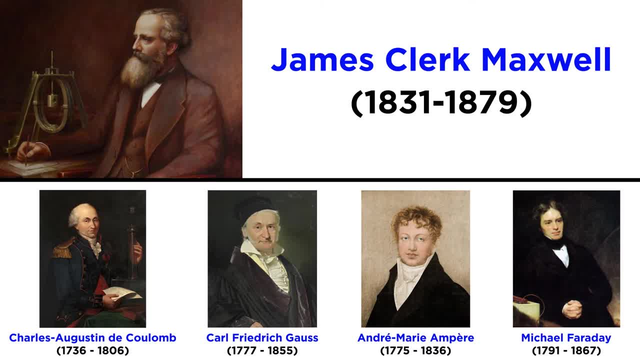 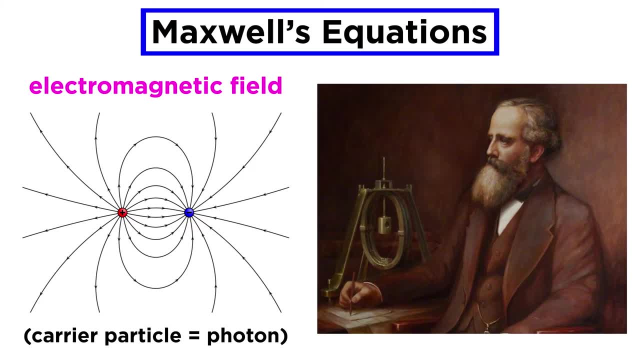 years of work by earlier well-known scientists, those being Coulomb, Gauss, Ampere and Faraday. Formulated almost two hundred years ago, they are still the simplest way to accurately represent laws of the electromagnetic field and its carrier particle, the photon. Each of these 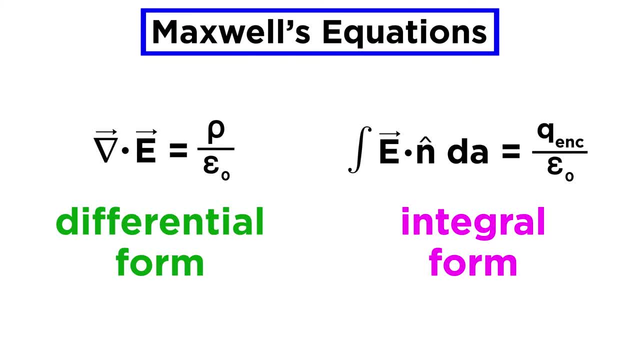 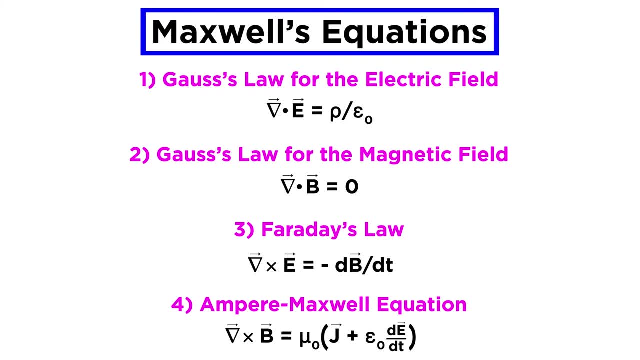 four equations, has two forms: a differential form and an integral form. We are going to examine Maxwell's four equations, one at a time, over the next four tutorials. The first one is Gauss's law for the electric field. so let's start with the foundational concepts. 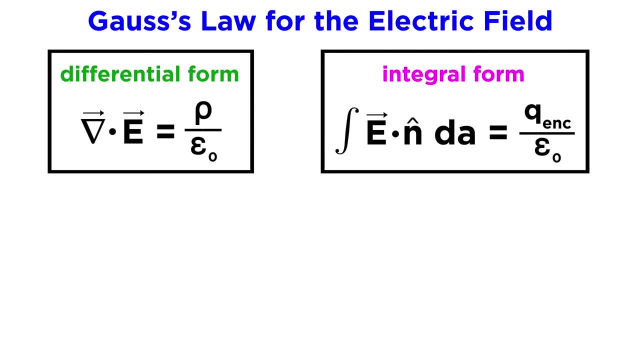 behind the derivation of this law. As we mentioned, this law has both differential and integral forms. These two forms are called differential and integral. The differential and integral forms are useful in entirely separate situations. The differential form states that the divergence of the electric field in a given region is related to the charge density within that. 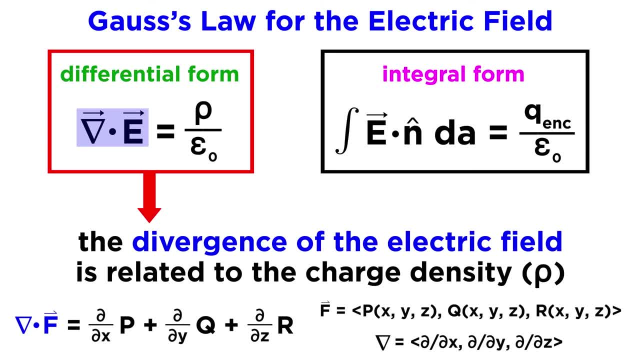 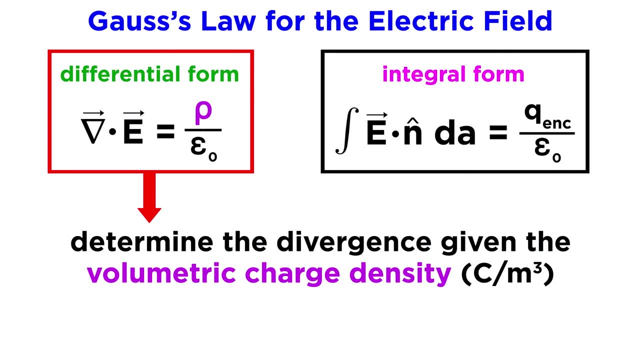 region. Remember that divergence means we are finding this dot product where the del operator is a vector comprised of the relevant partial differential operators, and that the divergence of a vector field, like this electric field, gives us a scalar field. The differential form is used to determine the divergence of an electric field at a particular point. 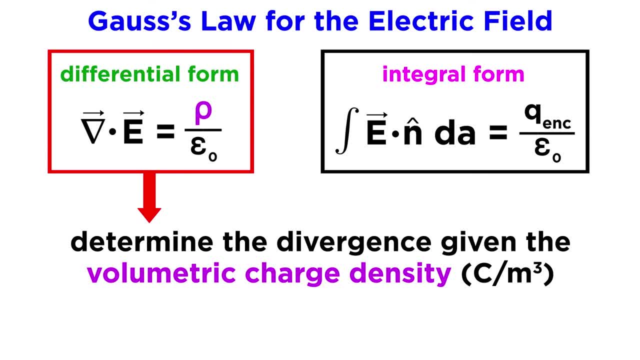 if the volumetric charge density rho is known, meaning the quantity of charge per unit volume measured in coulombs per cubic meter. Epsilon naught is a constant representing the permittivity of free space or the capability of a vacuum to permit electric fields. Conversely, 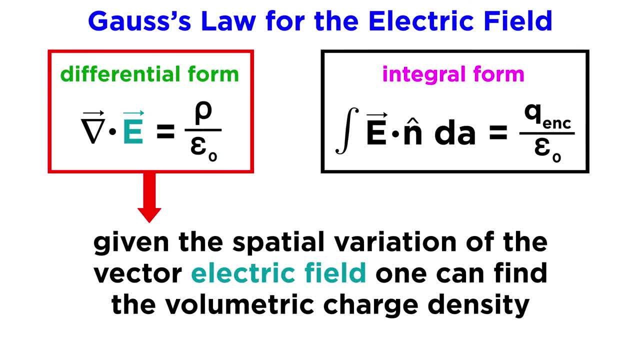 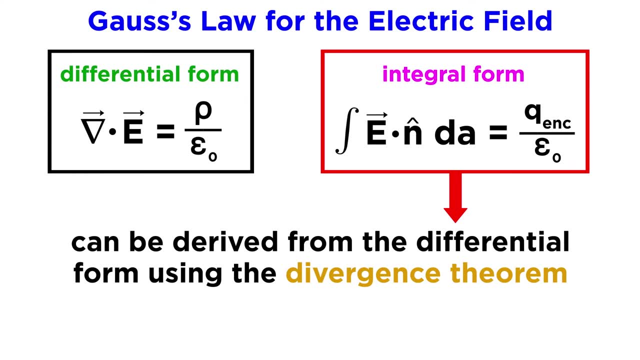 the permittivity of free space or the capability of a vacuum to permit electric fields. Conversely, differential form allows us to find the volumetric charge density at a particular point. The integral form can be derived directly from the differential form by applying the divergence theorem. 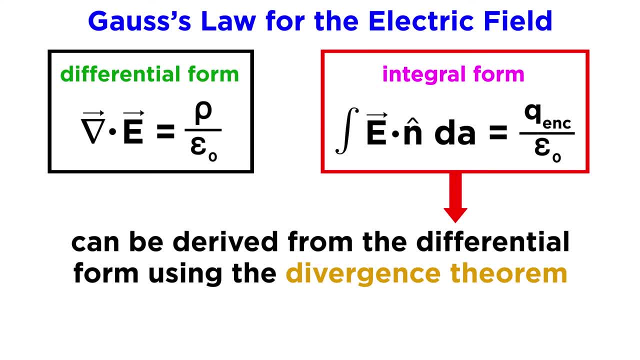 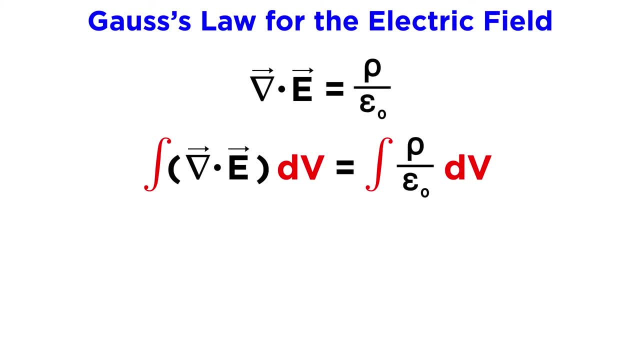 which we went over in one of the mathematics tutorials. Let's quickly run through the derivation together. First, we will take the differential form and integrate both sides with respect to dv, which is the differential volume, essentially the same as dx, dy, dz in Cartesian. 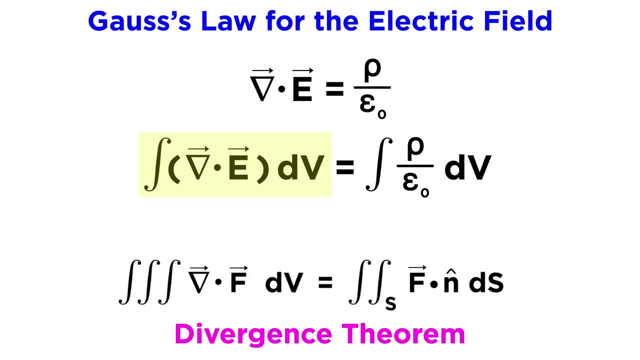 space. Now, the left side of this equation resembles one side of the divergence theorem. This theorem says that the triple integral of the divergence of a vector field, which is what is represented here, given the del operator and the fact that we are integrating with respect to dv. 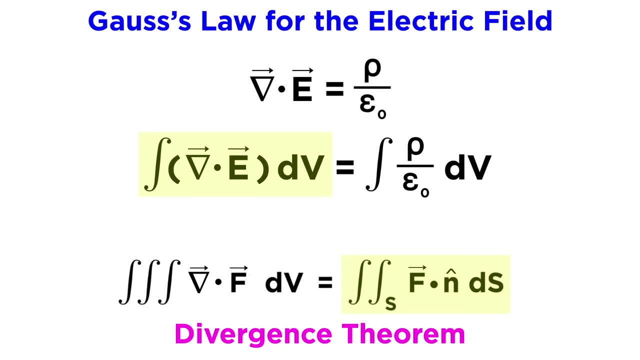 is equal to this surface integral. So we can change what we have to this surface integral and for our purposes we can simply express it in this way, because the electric field is the function of the factor. So we can simply express the electric field in this way, because the 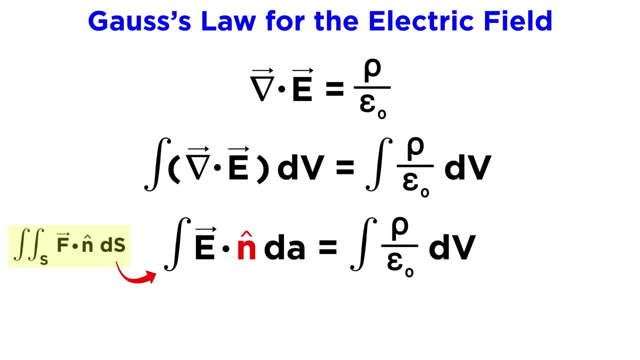 force. in this situation, N hat is the normal unit vector, as we would expect, and then dA is the integrand for this surface integral that will allow us to express it as a single integral. Then the final step is to reduce the integral on the right side, Knowing that 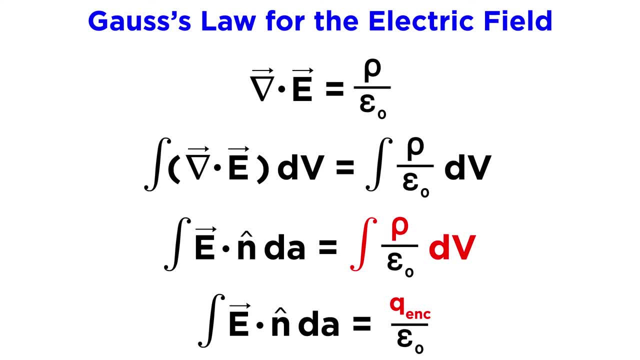 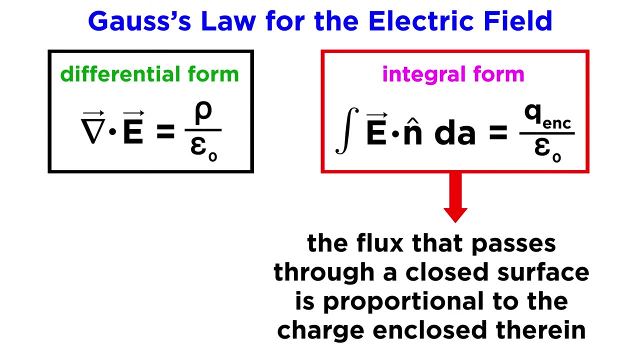 epsilon naught is a constant and the charge density rho, taken over the entire enclosed volume, is simply the enclosed charge Q. that will leave us with this, And there we have the integral form of this law. This form states that the flux passing through 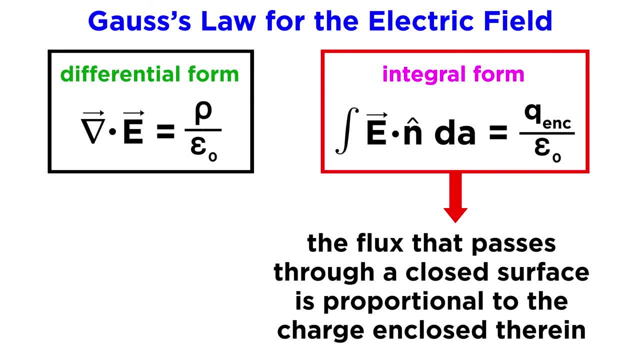 a closed surface is proportional to the charge enclosed therein. The flux of an electric field can be thought of as analogous to the amount of fluid flow through an imaginary flat surface. This equation can be used to determine the flux of an electric field from the enclosed charge or the total enclosed charge from the flux, Unlike the differential, 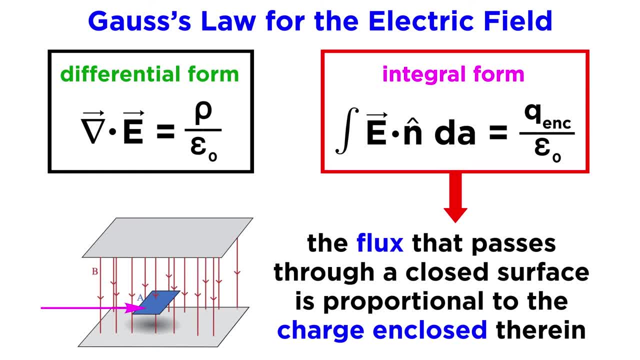 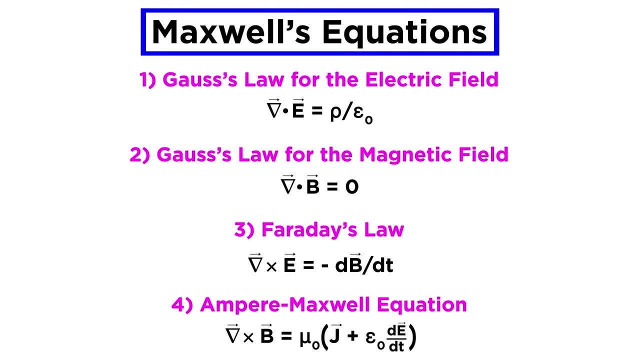 form. the integral form acts over a surface area. Now, each of Maxwell's equations describes the electromagnetic field in a different way. They are tailored to meet the requirements of a certain problem set in the real world. Gauss's law for the electric field excels. 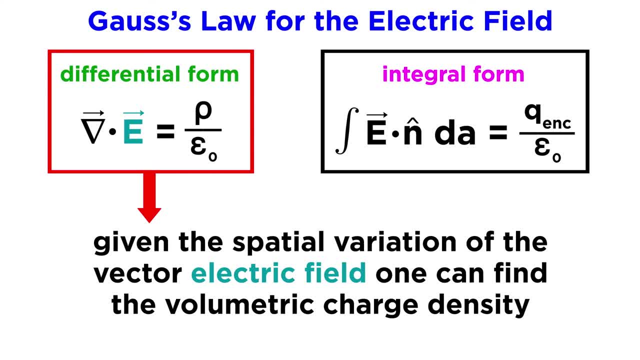 if the spatial variation of the vector electric field is known, then the differential form of the vector field is known and the density of charge density is known. This form is used to determine the divergence of an electric field at a particular point. if the volumetric charge density 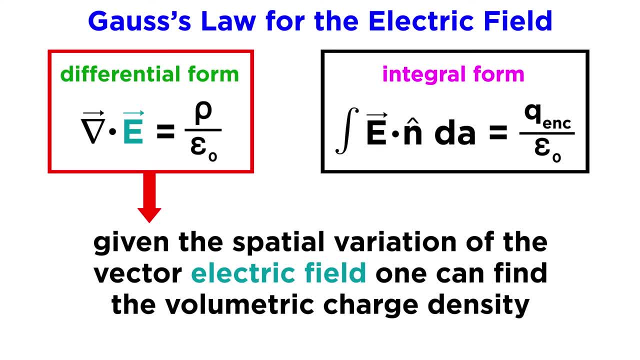 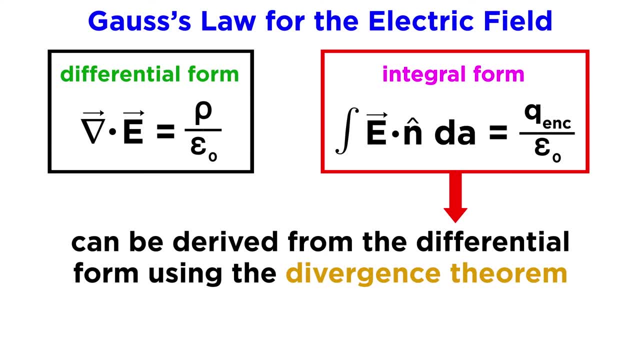 the differential form allows us to find the volumetric charge density at a particular point. The integral form can be derived directly from the differential form by applying the divergence theorem, which we went over in one of the mathematics tutorials. Let's quickly run through the derivation together. First we will take the differential form and integrate. 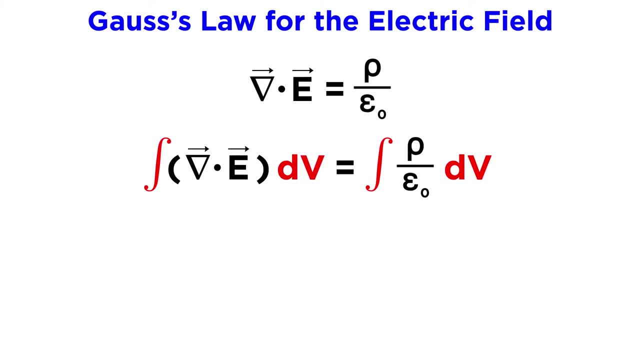 both sides with respect to dv, which is the differential volume, essentially the same as dx, dy, dz in Cartesian space. Now, the left side of this equation resembles one side of the divergence theorem. This theorem says that the triple integral of the divergence of a vector field, which is what is represented, 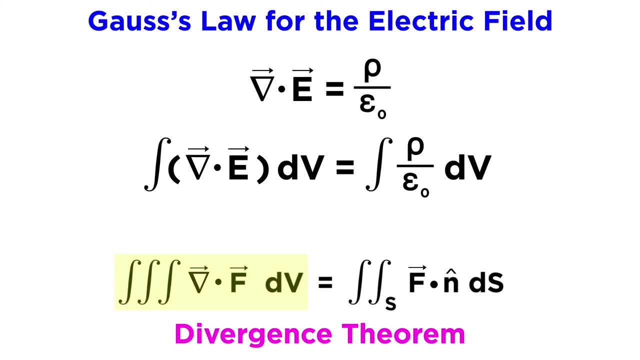 here, given the del operator and the fact that we are integrating with respect to dv, is equal to this surface integral. So we can change what we have to this surface integral and for our purposes we can simply express it in this way, because the electric field 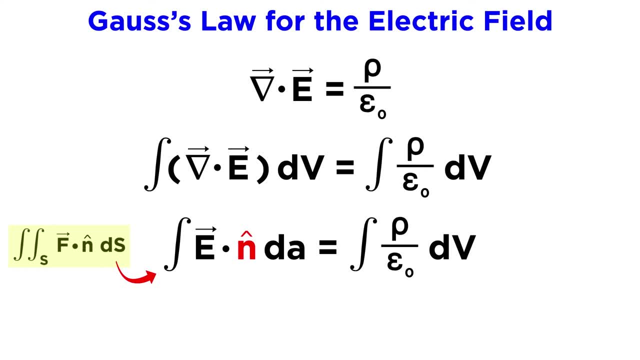 is the force in this situation. So we can simply express it in this way: because the electric field is the force in this situation, n hat is the normal unit vector, as we would expect, and then dA is the integrand for this. 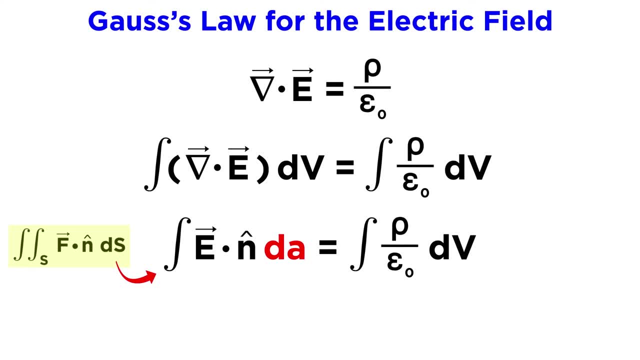 surface integral that will allow us to express it as a single integral. Then the final step is to reduce the integral on the right side, Knowing that epsilon naught is a constant and the charge density rho taken over the entire enclosed volume is simply the enclosed. 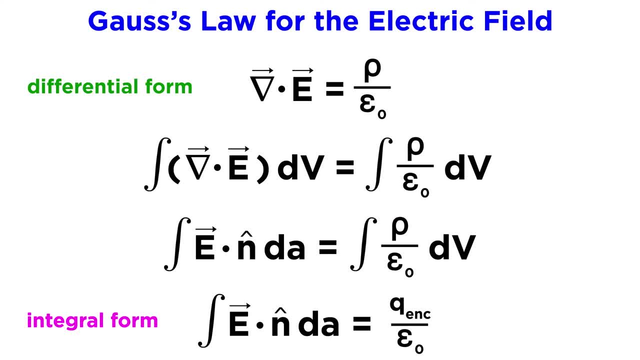 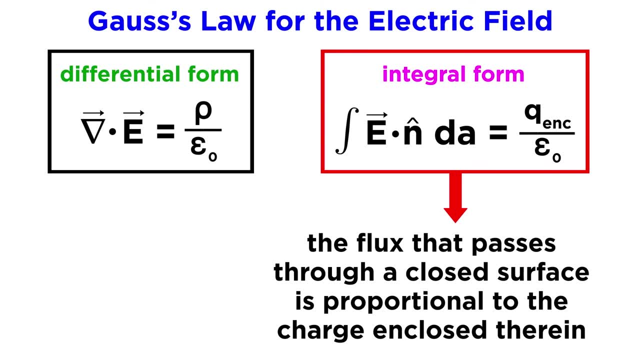 charge Q. that will leave us with this, And there we have the integral form of this law. This form states that the flux passing through a closed surface is proportional to the charge enclosed therein. The flux of an electric field can be thought of as: 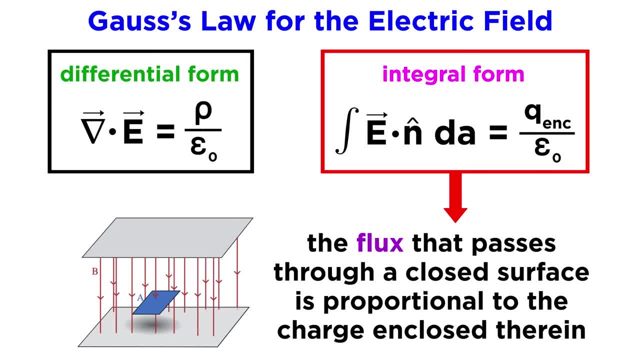 analogous to the amount of fluid flow through an imaginary flat surface. This equation can be used to determine the flux of an electric field from the enclosed charge or the total enclosed charge from the flux. Unlike the differential form, the integral form acts over a surface area. 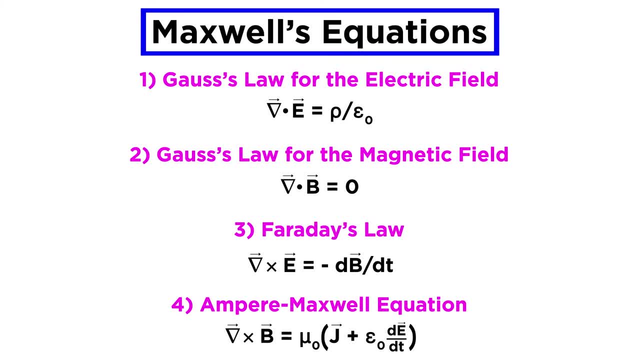 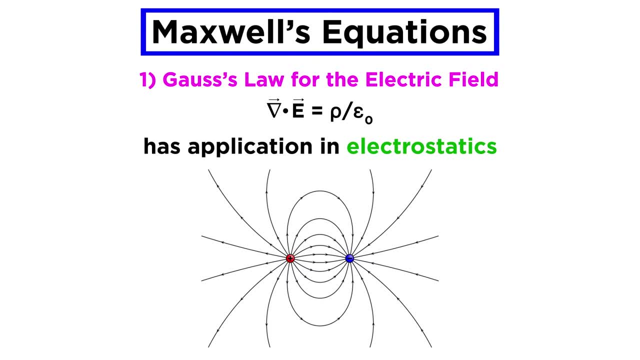 Now, each of Maxwell's equations describes the electromagnetic field in a different way. They are tailored to meet the requirements of a certain problem set in the real world. Gauss's law for the electric field excels in the realm of electrostatics, where all 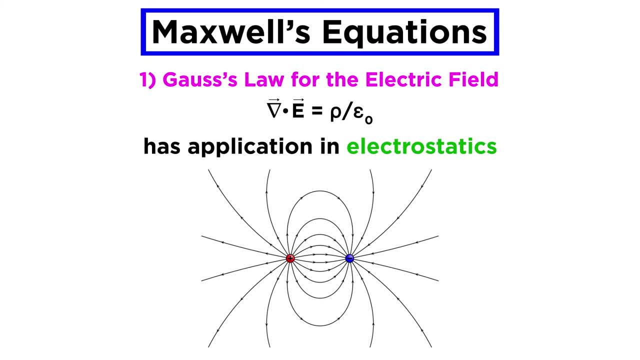 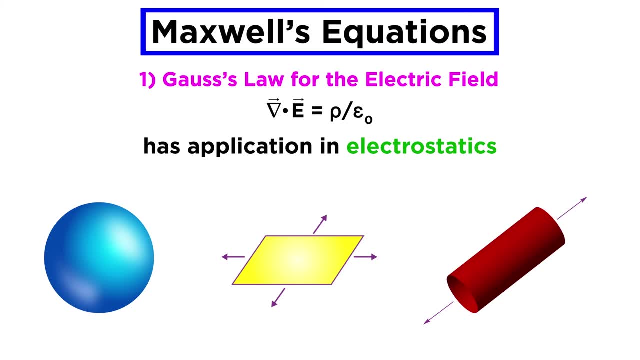 charges or charged objects are stationary and the boundary conditions are well known. For this reason, it is often the simplest starting point. The practice problems associated with this equation are often the same as the ones we have seen in the previous video, but they usually involve simpler shapes like spheres, infinite sheets and infinite cylinders. 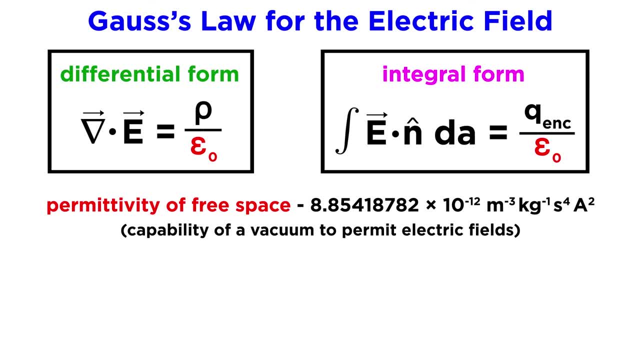 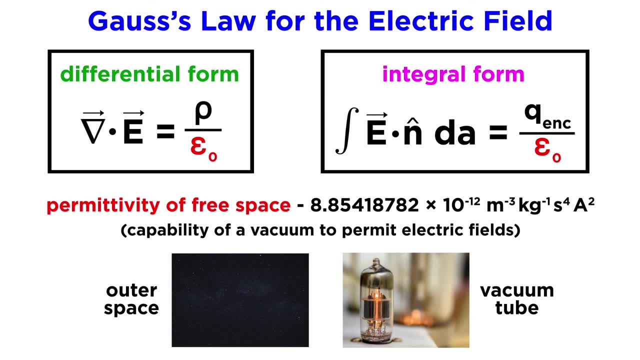 Let's look at the two forms of this law again. In both forms there is the constant we described earlier, the permittivity of free space. This constant is only valid for situations where all currents, both bound and free, are accounted for In a more approachable situation than 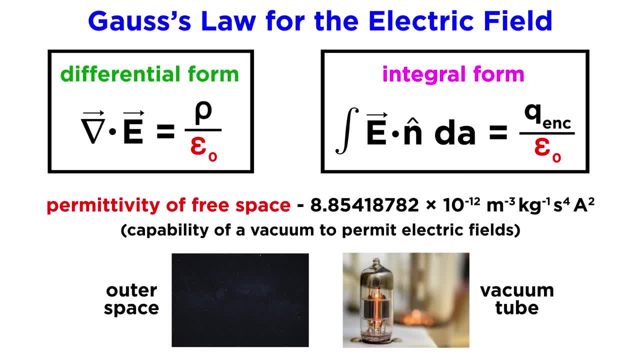 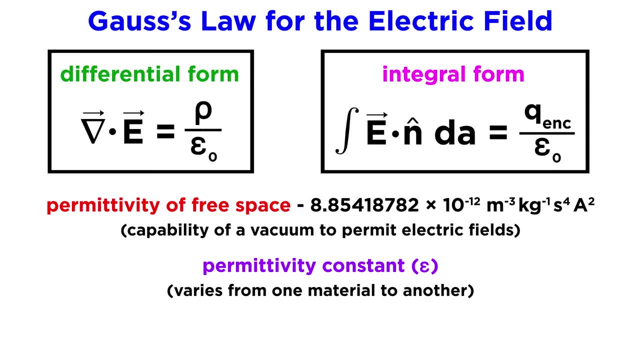 the vast emptiness of deep space or a large laboratory vacuum tube. this value is set by the material or materials that the electric field in question interacts with. In other words, the permittivity differs from one material to another, with free space acting as the. 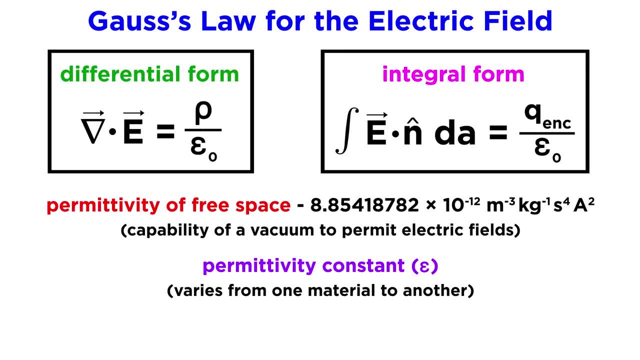 base line represented by epsilon naught, whereas epsilon without the naught will represent a permittivity constant for a specific material, and we can define the vector field D in this manner as the electric field times permittivity. In such a scenario, Gauss's law can be expressed in this manner: where the permittivity constant. 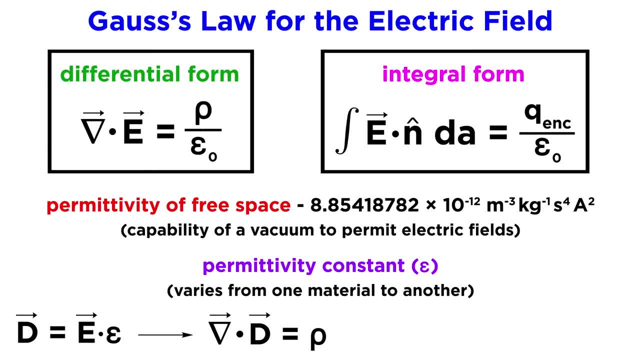 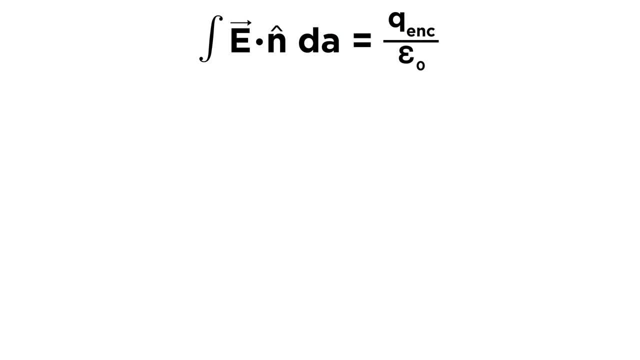 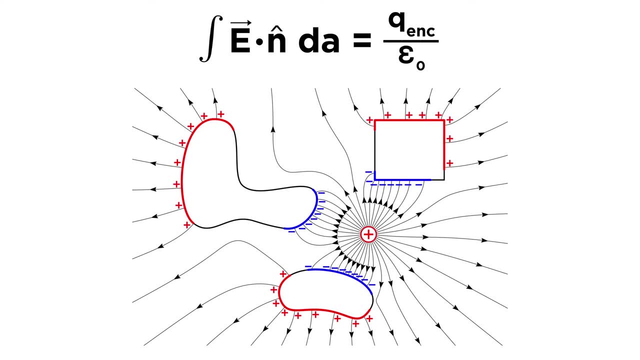 constant is not shown because it is accounted for in D. The same goes for the corresponding integral form. Now let's apply this understanding to solve a problem. Consider the integral form of Gauss's law. Finding the electric field from a given charge distribution may seem a daunting if 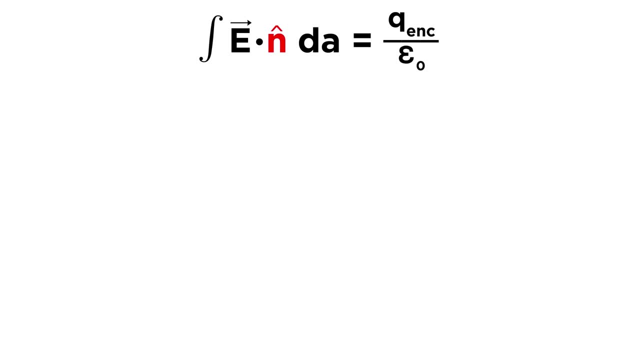 not impossible task. From the dot product, only the normal component emerges, leaving the electric field term trapped within the integral. There exists a very limited set of scenarios, all characterized by a high degree of symmetry, that allow us to both remove the electric field from the integral and simplify the dot product into simple algebraic. 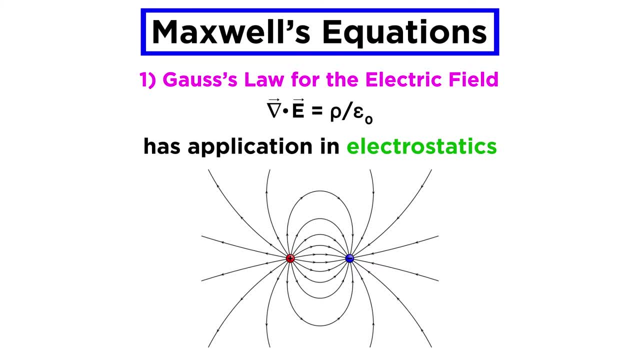 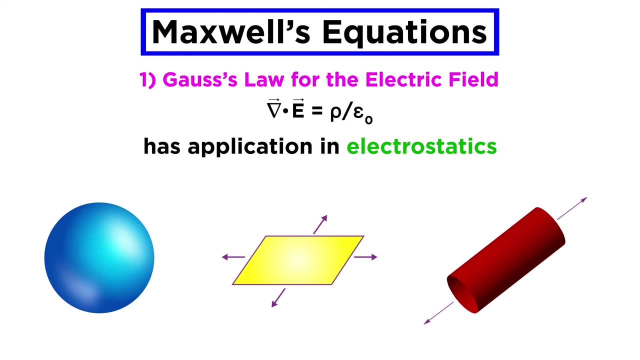 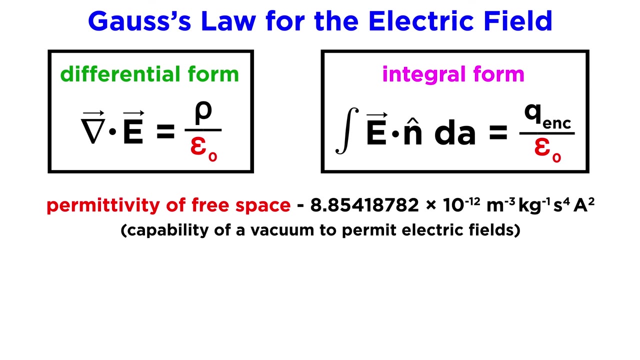 in the realm of electrostatics, where all charges or charged objects are stationary and the boundary conditions are well known. For this reason, it is often the simplest starting point. The problems associated with this equation usually involve simpler shapes like spheres, infinite sheets and infinite cylinders. Let's look at the two forms of this law again. 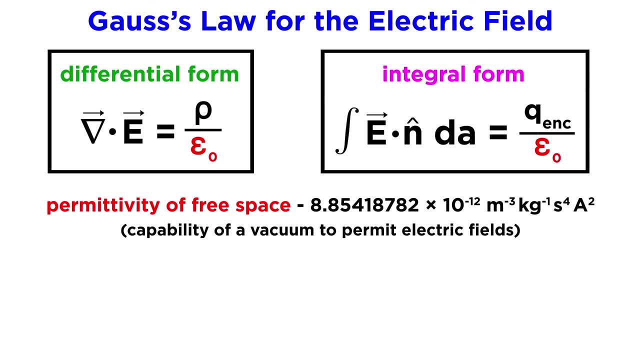 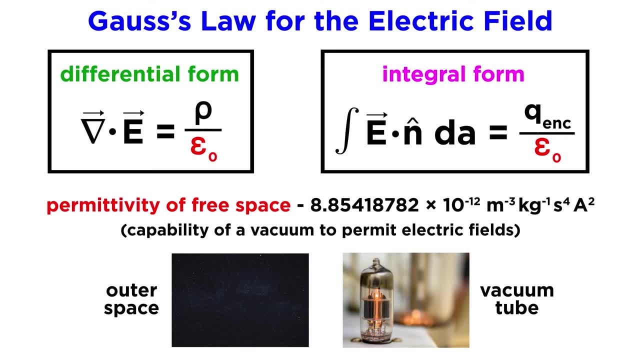 In both forms. there is the constant we described earlier, the permittivity of free space. This constant is only valid for situations where all currents, both bound and free, are accounted for In a more approachable situation than the vast emptiness of deep space or a large 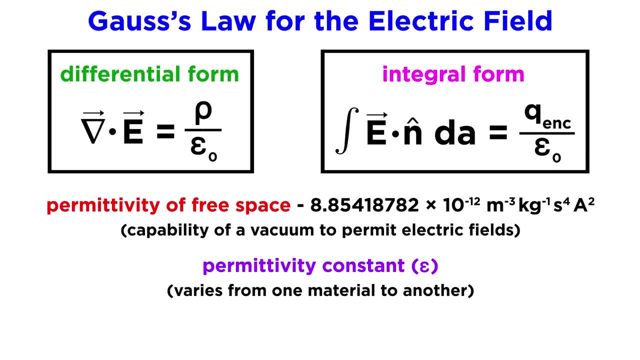 laboratory vacuum. the constant is only valid for situations where all currents, both bound and free, are accounted for In a more approachable situation than the vast emptiness of deep space or a large laboratory vacuum. this value is set by the material or materials. 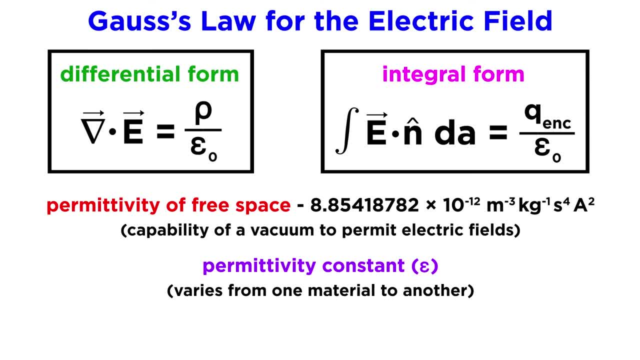 that the electric field in question interacts with. In other words, the permittivity differs from one material to another, with free space acting as the baseline represented by epsilon naught, whereas epsilon without the naught will represent a permittivity constant. for. 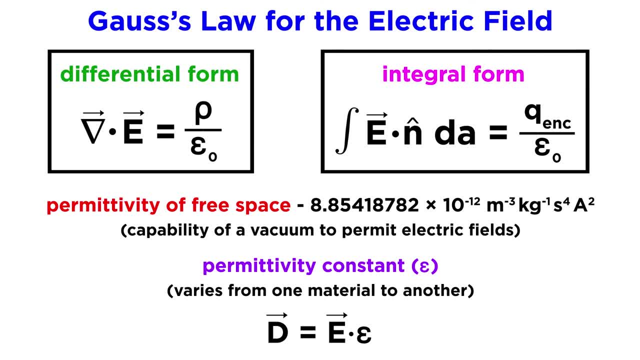 a specific material, and we can define the vector field d in this manner as the electric field times permittivity. In such a scenario, Gauss's law can be expressed in this manner: where the permittivity constant is not shown because it is accounted for. 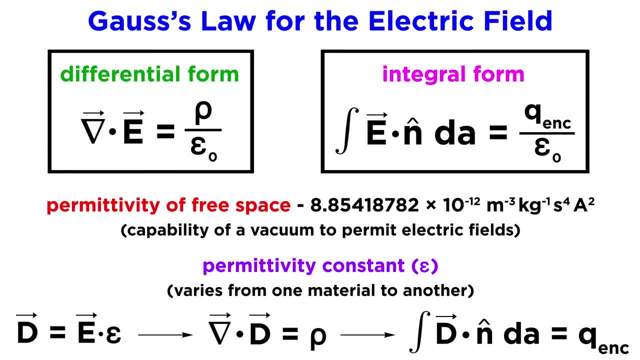 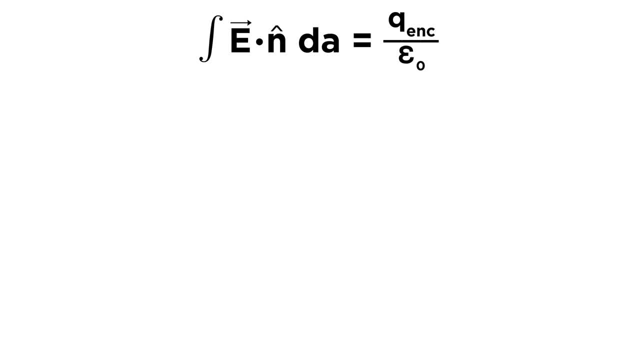 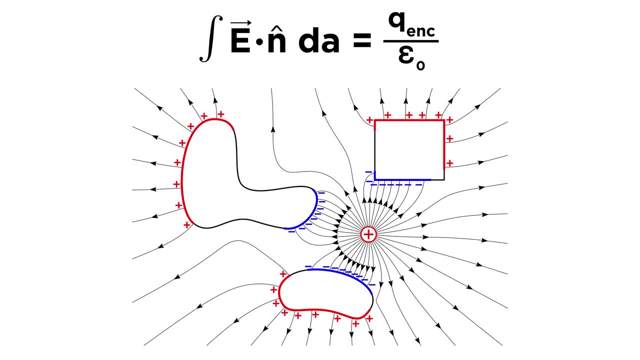 in d. The same goes for the corresponding integral form. Now let's apply this understanding to solve a problem. Consider the integral form of Gauss's law. Finding the electric field from a given charge distribution may seem a daunting, if not impossible task. From the dot product, only the normal component emerges, leaving 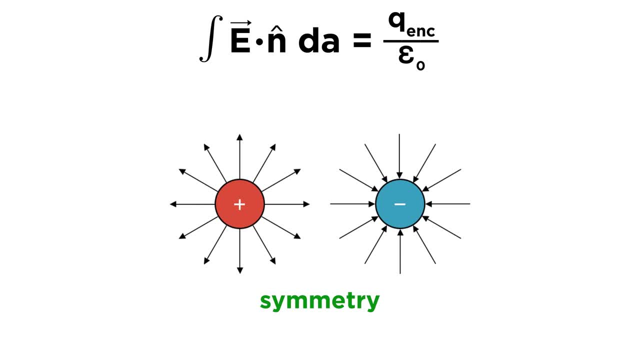 the electric field term trapped within the integral. There exists a very limited set of scenarios, all characterized by a high degree of symmetry, that allow us to both remove the electric field from the integral and simplify the dot product into simple algebraic multiplication. Thus, with Gauss's law for the electric field, 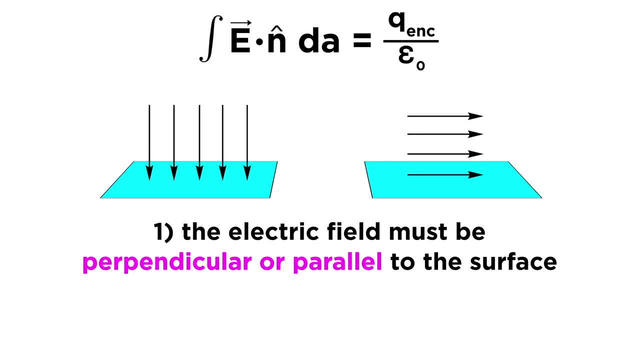 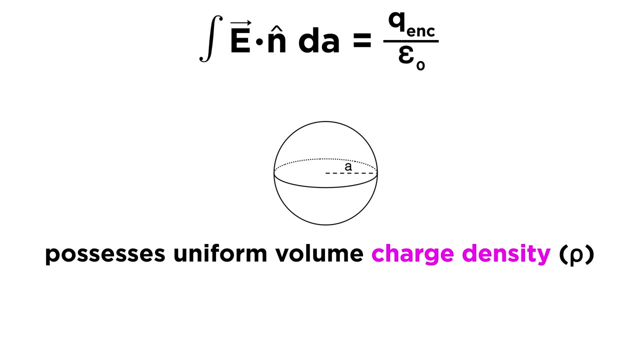 the electric field must be perpendicular or parallel to the surface and the electric field must be a constant or zero over the surface. Let's solve a problem that meets these conditions. Suppose there is a small charged sphere in space with a uniform volume, charge density, rho and radius. 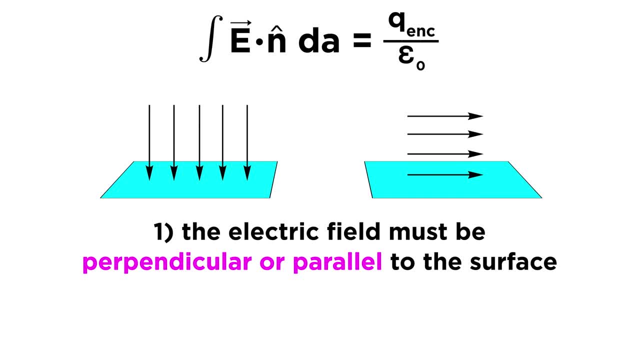 multiplication. Thus, with Gauss's law for the electric field, the electric field must be perpendicular or parallel to the surface and the electric field must be a constant or zero over the surface. Let's solve a problem that meets these conditions. Suppose there is a small charged. 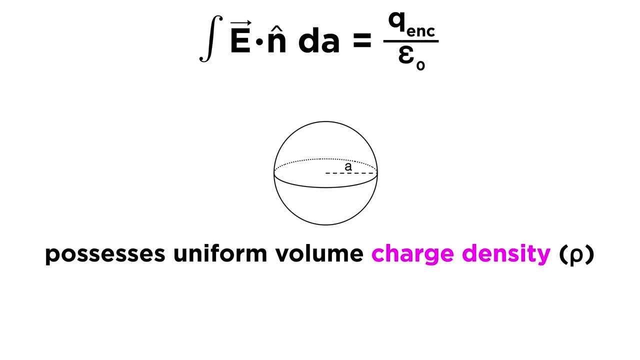 sphere, We need to find the electric field at a distance r from the center of the charged sphere. To do this, we must create a special Gaussian surface around the charged sphere. This surface has to meet the two criteria we mentioned before, and a sphere of radius r will do it. 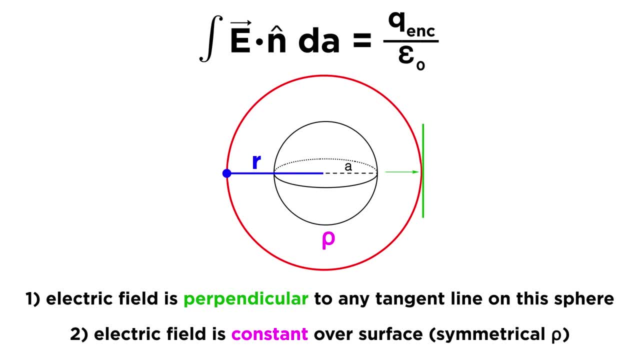 The electric field will be perpendicular to the surface and the electric field will be constant over the surface because the charge distribution inside the Gaussian surface is spherically symmetrical. We will then manipulate Gauss's law according to this particular situation. We can pull the electric field out of the integral because it's constant. 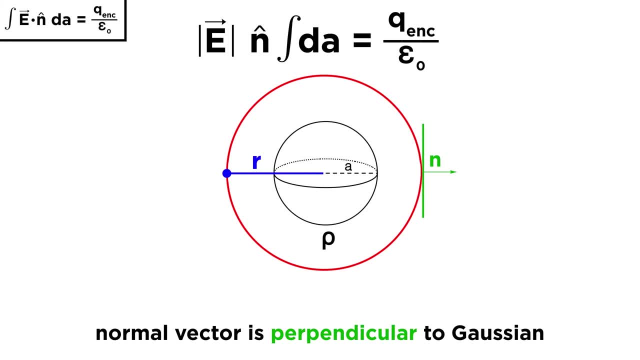 over the surface and we can pull the normal vector out of the integral because it is perpendicular to the surface of the Gaussian sphere and therefore reduces to one. Then we must integrate dA. This represents the surface area of the Gaussian sphere and the formula for the. 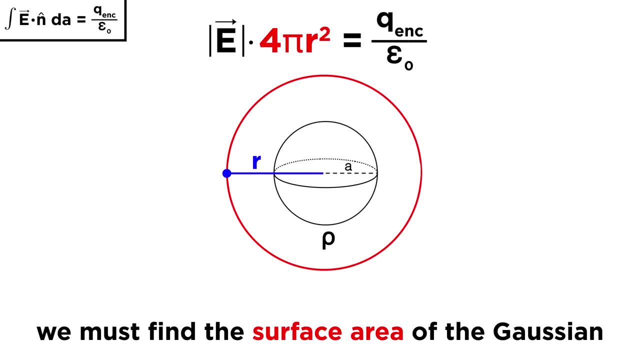 surface area of a sphere is four pi r squared. given that we have selected r as the radius for the Gaussian sphere, Then we can simply divide both sides by four pi r squared to solve for the electric field. Thus, the electric field will be equal to the total charge enclosed. 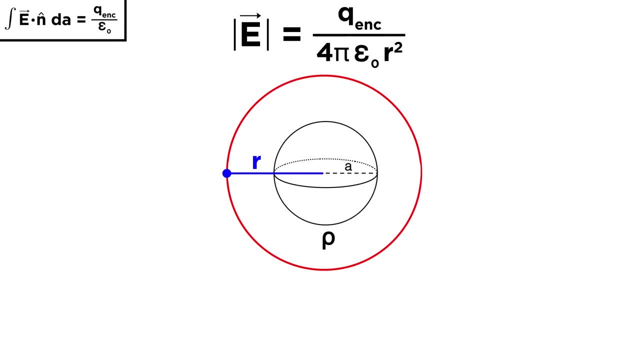 divided by the surface area of the sphere and the permittivity of free space. Let us notice that this is rather similar to Coulomb's law, which we introduced in a previous tutorial. In fact, if we acknowledge this value for k and make the substitution in Coulomb's law, 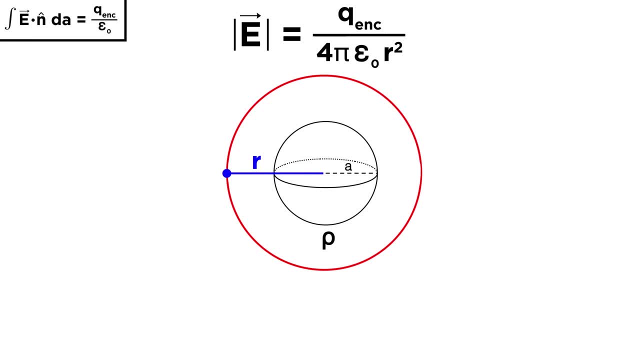 we see that they are nearly identical. We are not quite finished, however. The enclosed charge varies depending on the size of the chosen Gaussian sphere. Let us examine three scenarios. For the first scenario, if it is smaller than the charged sphere, meaning r. 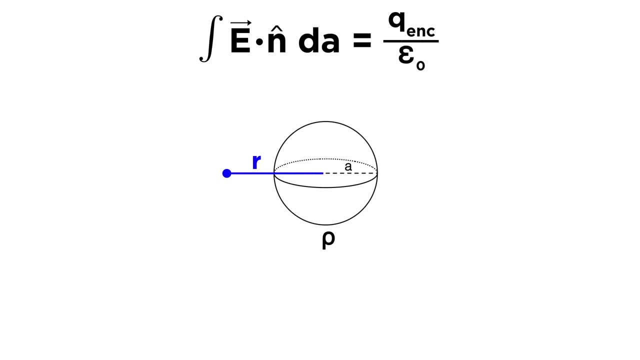 a. We need to find the electric field at a distance r from the center of the charged sphere. To do this, we must create a special Gaussian surface around the charged sphere. This surface has to meet the two criteria we mentioned before: and a sphere of radius. 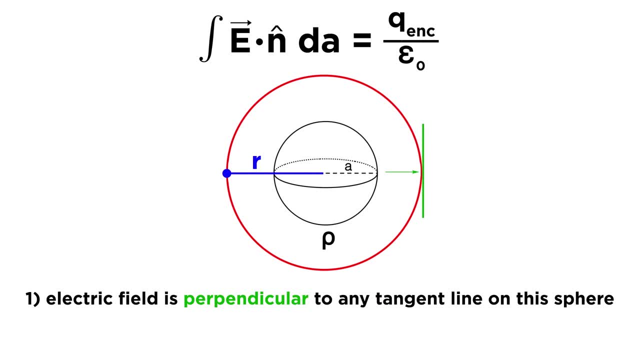 r will do it. The electric field will be perpendicular to the surface and the surface will be at the center of the charged sphere. To solve this, we are to use R. To solve R, we must use the constant formula. A free solution is a constant. 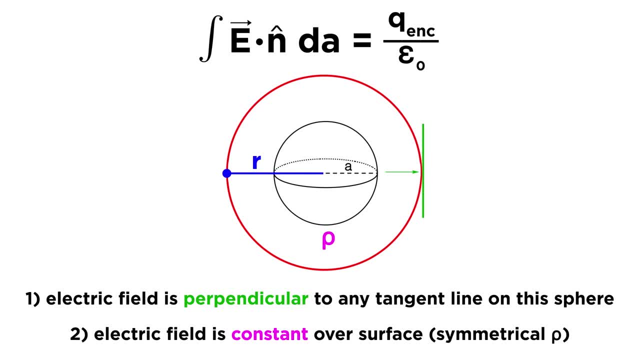 volume, charge density, rho and radius a. This surface has to meet the two criteria we mentioned. surface and the electric field will be constant over the surface because the charge distribution inside the Gaussian surface is spherically symmetrical. We will then manipulate Gauss's law according to this particular situation. 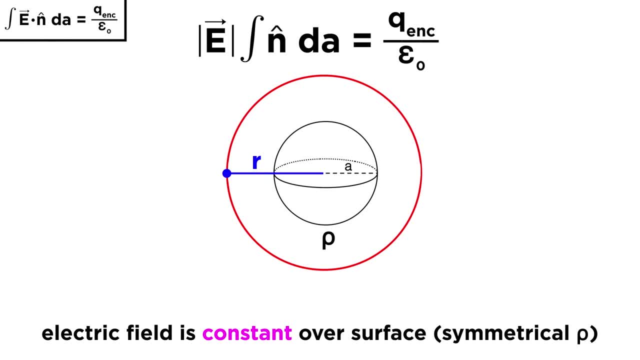 We can pull the electric field out of the integral because it's constant over the surface, and we can pull the normal vector out of the integral because it is perpendicular to the surface of the Gaussian sphere and therefore reduces to one. Then we must integrate dA. 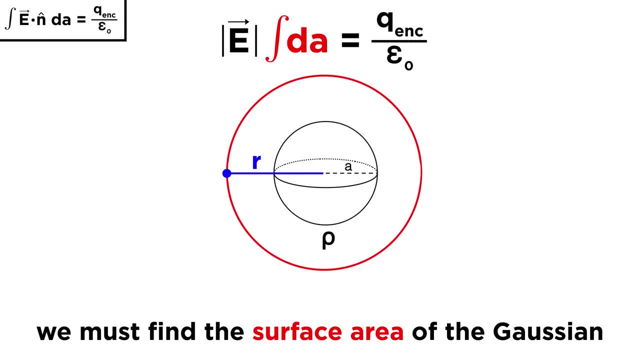 This represents the surface area of the Gaussian sphere, and the formula for the surface area of a sphere is four pi r squared. given that we have selected r as the radius for the Gaussian sphere, Then we can simply divide both sides by four pi r squared to solve for the electric field. 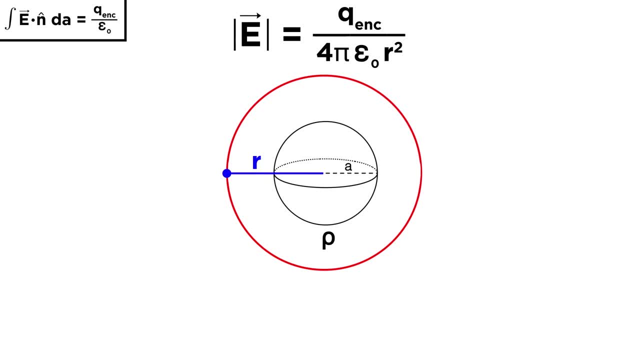 Thus, the electric field will be equal to the total charge enclosed, Divided by the surface area of the sphere and the permittivity of free space. Let us notice that this is rather similar to Coulomb's law, which we introduced in a previous tutorial. 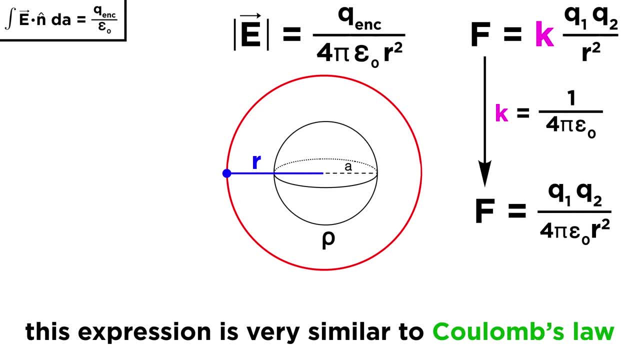 In fact, if we acknowledge this value for k and make the substitution in Coulomb's law, we see that they are nearly identical. We are not quite finished, however. The enclosed charge varies depending on the size of the chosen Gaussian sphere. Let us examine three scenarios. 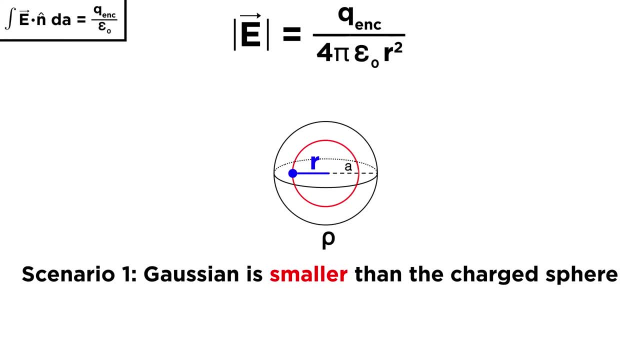 Let us examine three scenarios. For the first scenario, if it is smaller than the charged sphere, meaning r is less than a, then we can actually say that a equals r, because we will only be considering the charge density within the Gaussian. This means that q equals rho times the volume of the Gaussian, or four thirds pi r cubed. 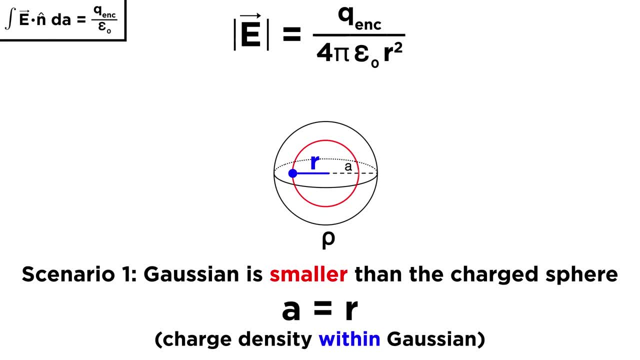 is less than a, then the charge will be equal to r squared. If it is smaller than the charged sphere, then we can actually say that a equals r, because we will only be considering the charge density. within the Gaussian. This means that q equals rho times the volume of 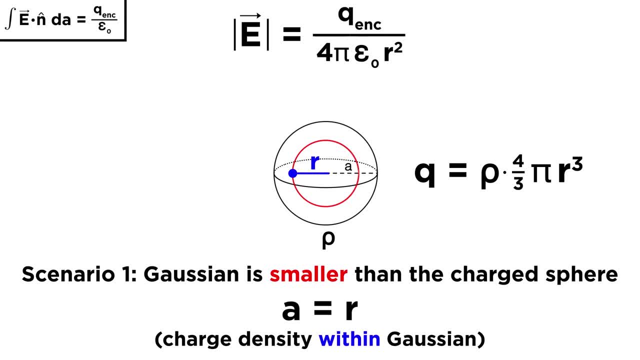 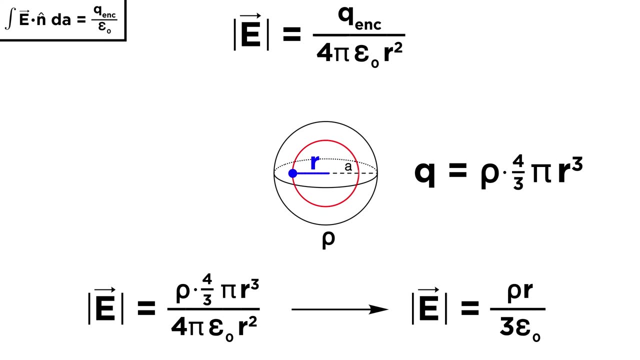 the Gaussian, or four thirds pi r cubed. We can plug this into our previous expression and we will see that four will cancel, pi will cancel and two of the r terms will cancel. The electric field would then simplify to this expression. For the second scenario, 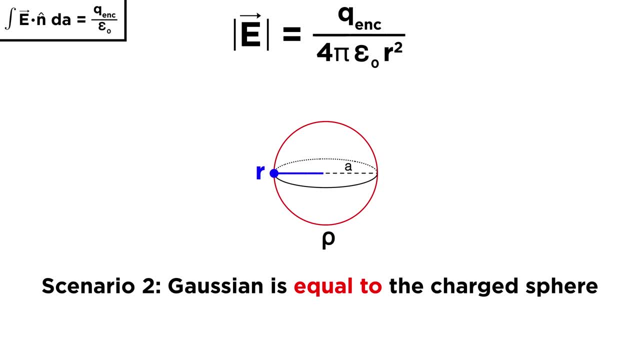 if we were to expand the Gaussian sphere so that it was exactly the same size as the charged sphere, such that r equals a, we would maximize the electric field as follows: by simply swapping r for a. For the third and final scenario, let's move our Gaussian sphere back outside the charged 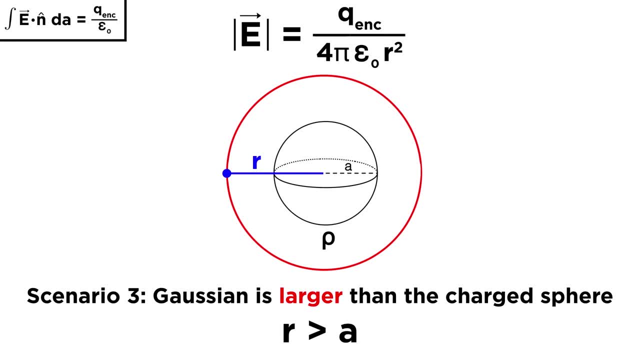 sphere such that r is greater than a. The enclosed charge would now be a constant, but the distance, r, would continue to increase. Thus we have this expression for Q with A in it, and that leaves us with this, which is essentially the same as the previous situation, except that the R's don't cancel, and. 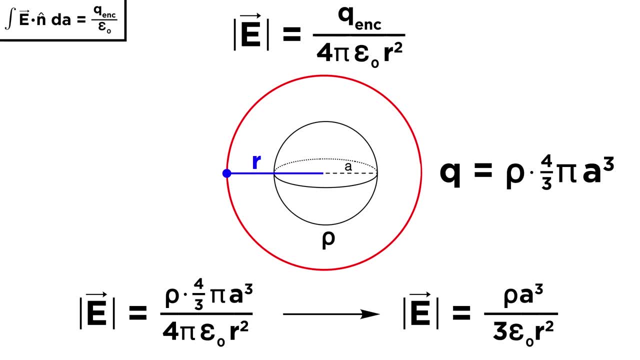 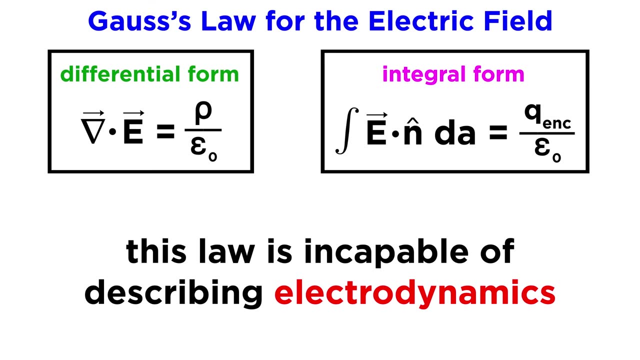 we are left instead with A cubed on top. Any of these expressions we have just derived can then be easily evaluated to calculate the electric field, And that gives us a picture of what we can calculate with this law. On its own, Gauss's law is not capable of interpreting the changing, shifting world. 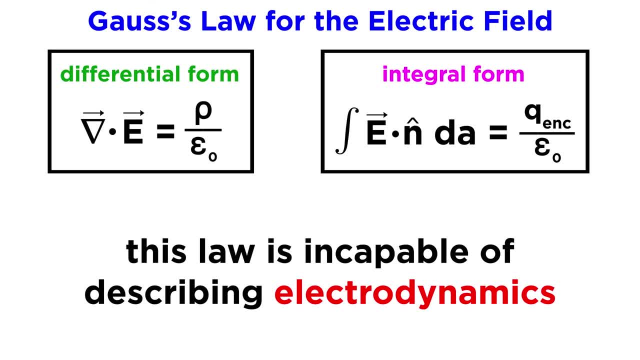 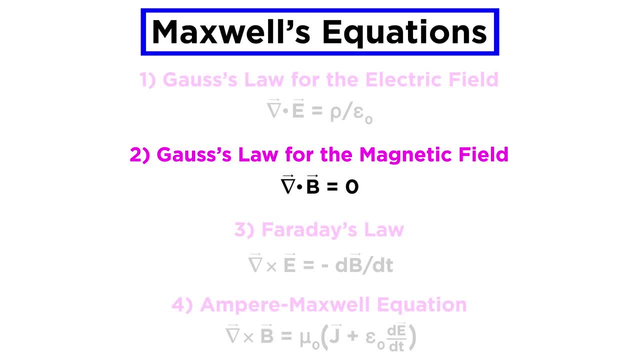 of electrodynamics that we inhabit. It is an incomplete picture tailored to a static, tightly controlled scenario. In the next tutorial we will cover the magnetic side of Gauss's law. This second of Maxwell's equations will complete the static picture of electromagnetism. 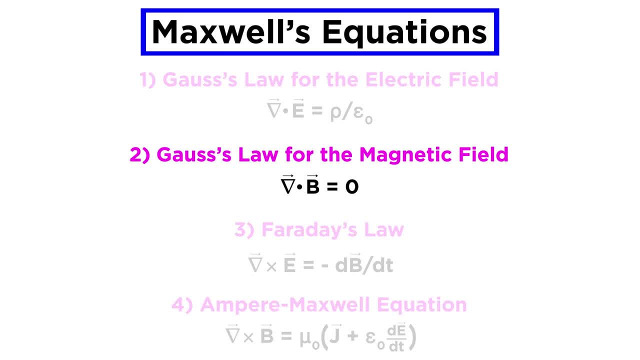 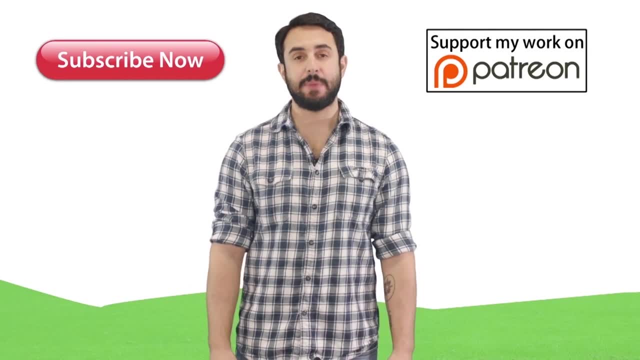 and lay the foundation for interpreting the dynamics of our ever-changing world. I hope you enjoyed the tutorials. Support me on Patreon so I can keep making content and, as always, feel free to email me professordaveexplains at gmail dot com.